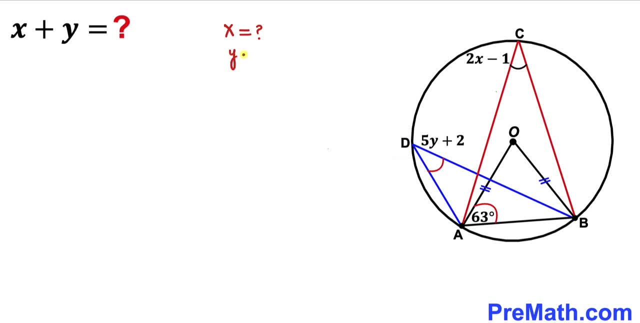 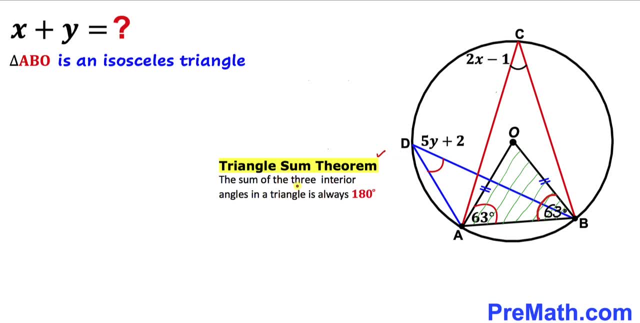 triangle sum theorem. according to this theorem, the sum of the three interior angles in a triangle is always equal to 180 degrees. So therefore, if this angle is 63 degrees, this angle is 63 degrees as well, So then this angle has got to be 54 degrees. If we add all these three angles, they 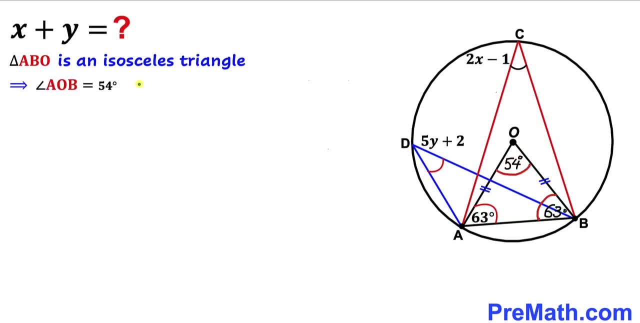 must add up to 180 degrees. So let's go ahead and solve for X plus Y. So let's go ahead and solve for X plus Y. So, therefore, if this angle is 64 degrees, this angle has got to be 64 degrees. So 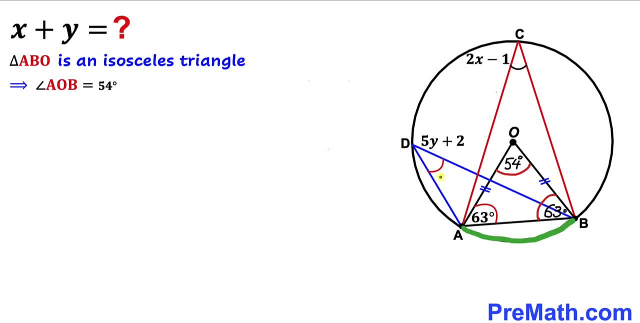 therefore, if this angle is 64 degrees, this angle has got to be 64 degrees. So let's go ahead and make an observation. We can see these three angles: this first angle, ADB, this angle ACB, and this, this angle, AOB, are subtended by this very same arc, AB And, moreover, this angle. 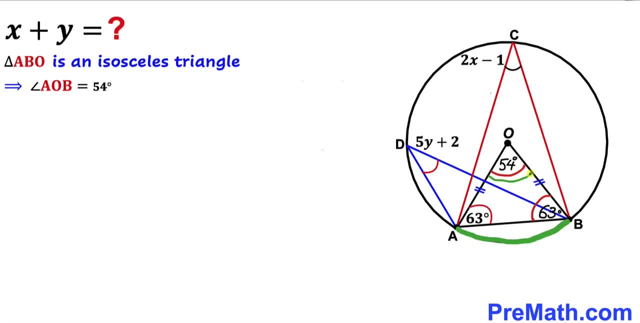 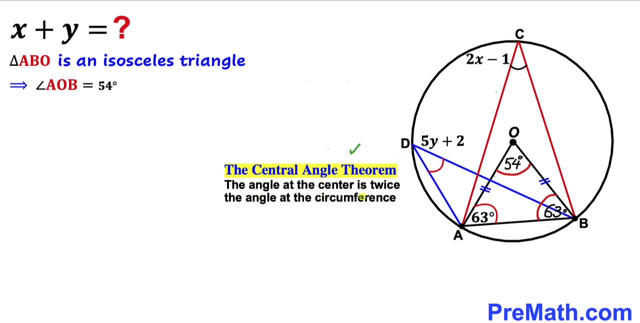 angle AOB is at the center, whereas these two angles, ADB and this angle ACB, are the angles at the circumference. and now let's recall the central angle theorem: the angle at the center is twice the angle at the circumference. so therefore this angle at the center AOB is going to be twice the angle at this. 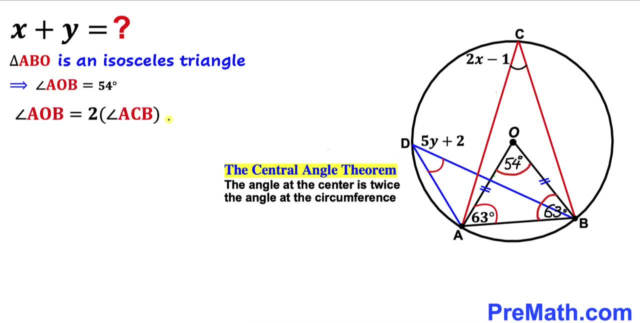 circumference ACB. therefore, we can write that this angle AOB equals to two times the angle ACB. we know our angle AOB is 54 degrees. let me go ahead and write down: 54 degrees equal to two times the angle ACB, is represented by 2x minus. 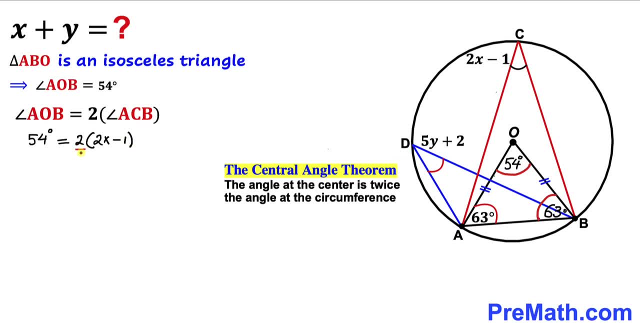 1. Now let's go ahead and divide both sides by 2, and on the left hand side, that is going to give us 27 degrees equal to this 2, let's go ahead and add one on both sides. this is gone. so therefore our number 2x. 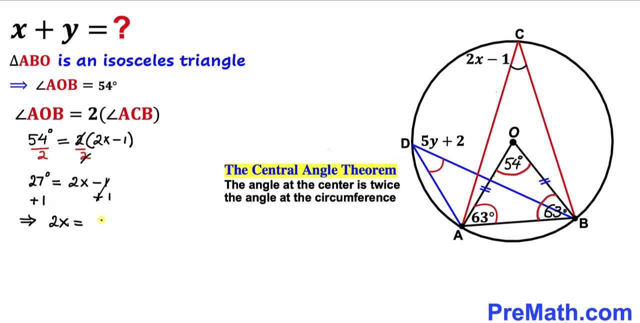 2x times 2b, raised by 1 times x, beats 2 everywhere. one minus index. x plus 1, be 27 plus 1 is going to make a 28, and let's divide both side by 2, so therefore our X value simply turns out to be 14 degrees. and here's our next step. now we 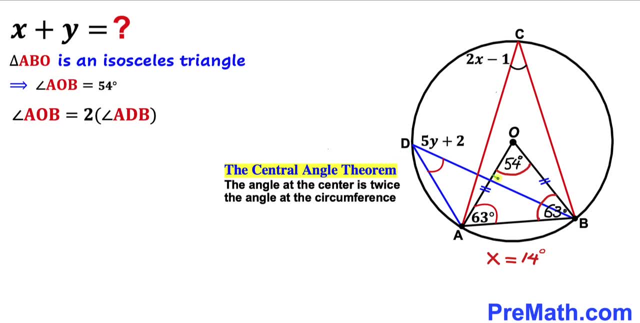 can see that this angle AOB at this center is twice of this angle ADB, as you can see over here in this equation, and we know our angle AOB is 54 degrees. therefore, let me go ahead write down: 54 degrees, equal to 2 times our angle ADB. 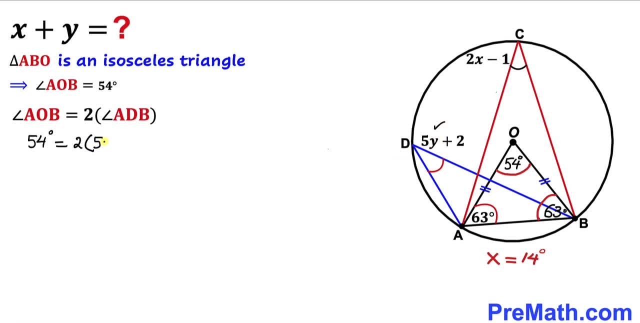 is represented by this 5y plus 2. let's go ahead and solve for y. so I'm going to divide both sides by 2 and we can see that this 2 and 2 is gone. on the left hand side, we got 27 degrees. 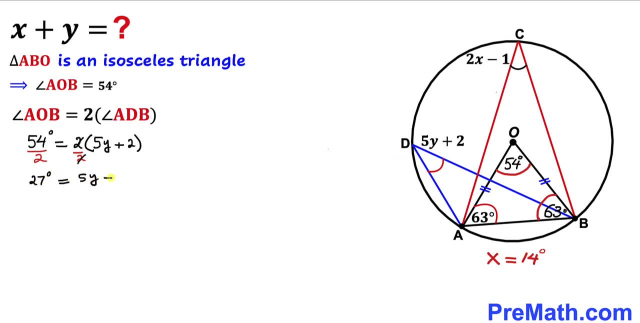 equal to 5y plus 2. let me go ahead and subtract 2 from both sides. this is gone. so therefore our 5y value turns out to be 25 degrees. so therefore our y value turns out to be 5 degrees. so thus we figured out. our x value is 14 degrees.